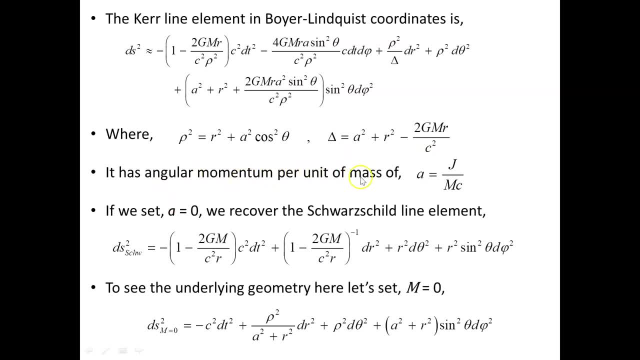 It has angular momentum, a rotating black hole, The Kerr rotating black hole is an angular momentum, a per unit of mass, sorry, angular momentum per unit of mass of j. So this is a recover the Schwarzschild line element which is this object here and you can see that coming from here. A goes to zero. a goes to zero, the cross term drops out, so it becomes really diagonal and highly symmetric in Delta. a goes to zero here and rho, the a bit disappears. so we get r over that. 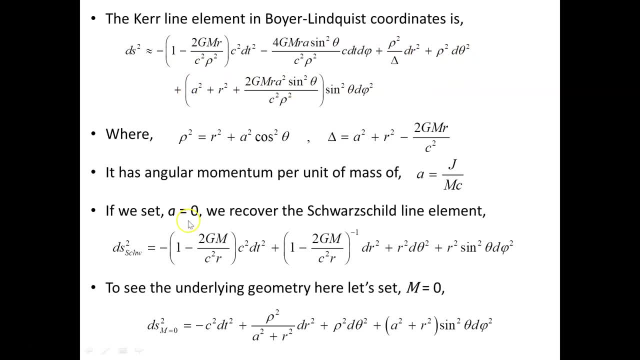 Ok, they're going to opposite sides and this becomes the Schwarzschild line element. If you go through bit by bit, you can see for yourself that that's the case. All right, Now to see the underlying geometry here. let's just remove M, set it to zero. 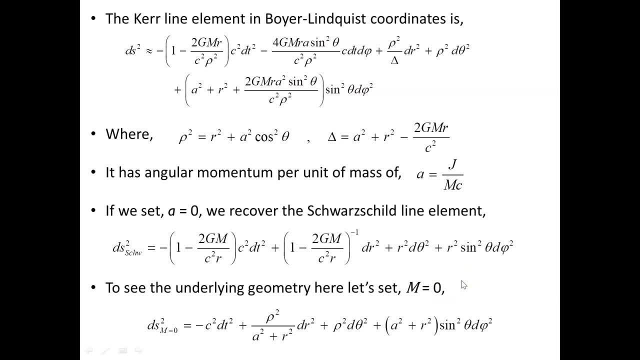 and we're not turning off the gravitational field, if you like, or anything like that. We just want to see what this looks like without the mass involved, And when we do that, we set M to zero. This again, cross term disappears here. 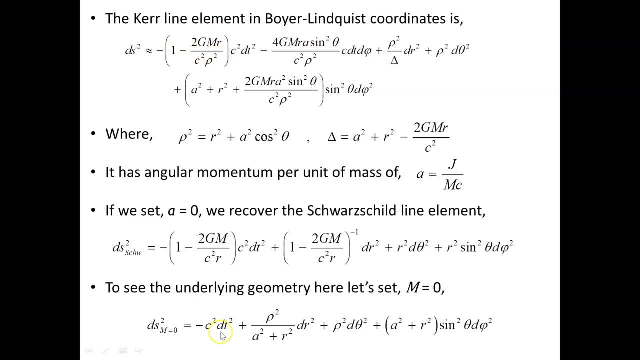 This bit disappears and becomes just minus one, And what we get is this object here, which we've seen before in a previous video on the derivation of the line element for Kerr geometry. But these coordinates here, if you like, elliptical coordinates, they're not spherical coordinates. 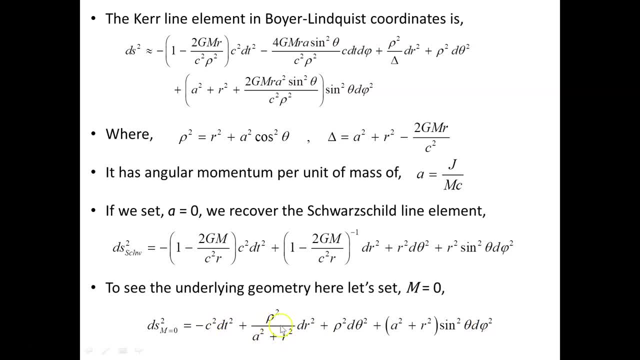 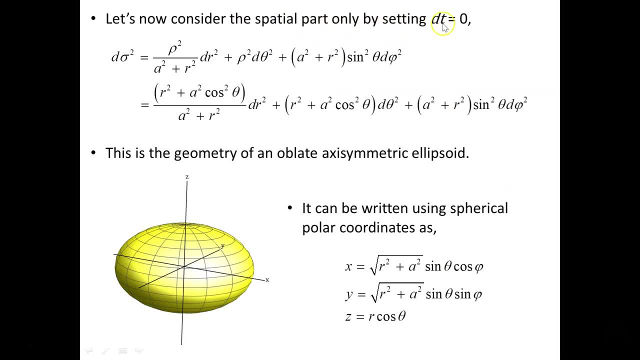 They don't describe a sphere, They describe an elliptical oblate, ellipsoid. Okay, So let's now consider spatial part only. We'll just set dt equal to zero and the hypersurface formed will be this, or the three surface will be this object here. 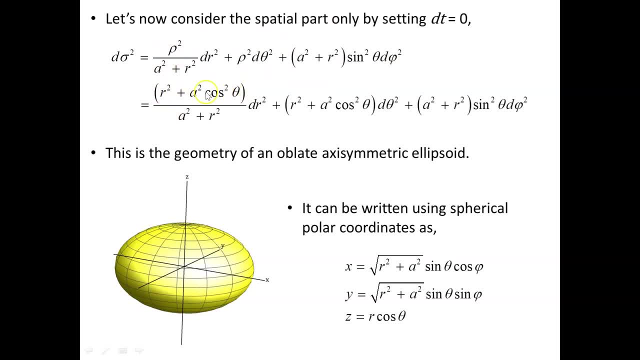 And we'll just get rid of the row there. write out its full expression and we have this object here Now. this is the geometry at oblate axisymmetric ellipsoid. The Z gets plus three Things such as pictured here. x and y have this extra a squared a factor in there, extra a squared term. 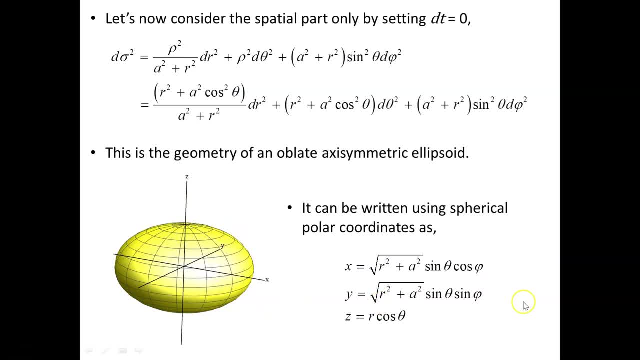 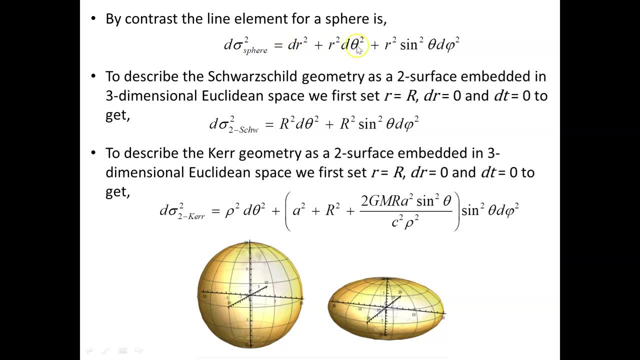 okay, and this gives us an oblate, axisymmetric ellipsoid. all right. by contrast, the line element for a sphere is this object here? okay, there's no a term in there. so that gives us a sphere. now to describe the schwarzschild geometry as a two surface embedded in three-dimensional euclidean space, we first set r equal to a. 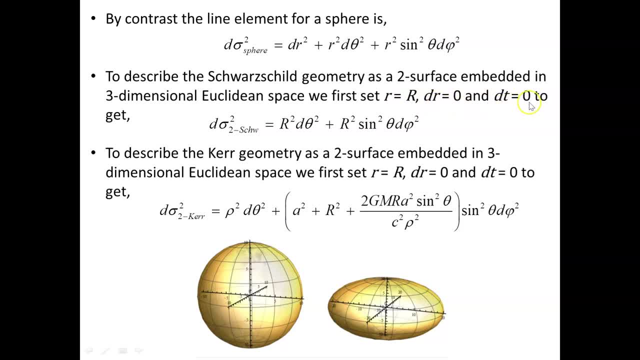 constant value, dr is zero and dt equals zero. to get the two surface formed by this d sigma squared, the line element d sigma squared for two surface- swatch type in the schwarzschild case- we get capital r squared d theta squared, plus capital r squared sine squared, theta d phi squared. 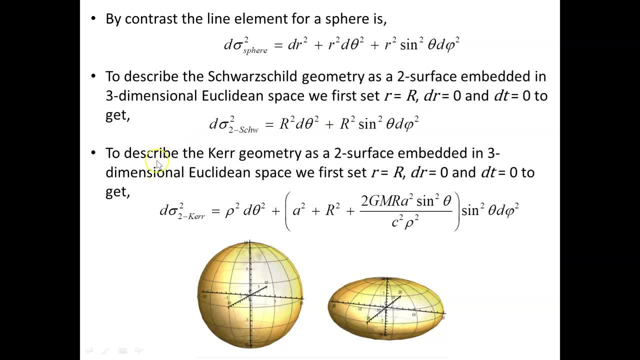 r is a constant. here capital r is a constant. okay, then we get a sphere that describes the surface of a sphere. all right, to describe the kerr geometry as a two surface embedded in three-dimensional euclidean space. so, as i hope, the surface two surface. first we set r equals capital r. again, dr is zero, dt is: 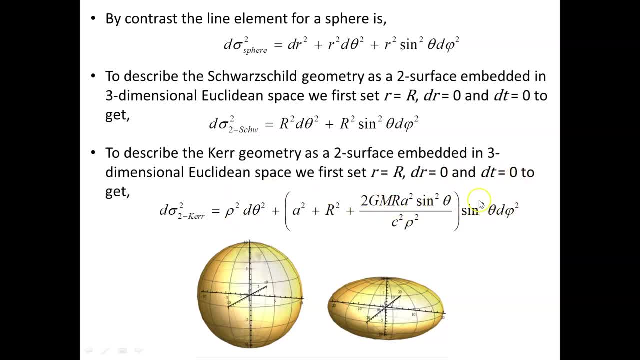 zero, again the same thing, and we produce this object here now. this is the line element of the surface describing the surface of this object here: an axisymmetric ellipsoid, very different to a sphere. okay, extended, dilated in the x and y directions. okay, flattened in the z direction. 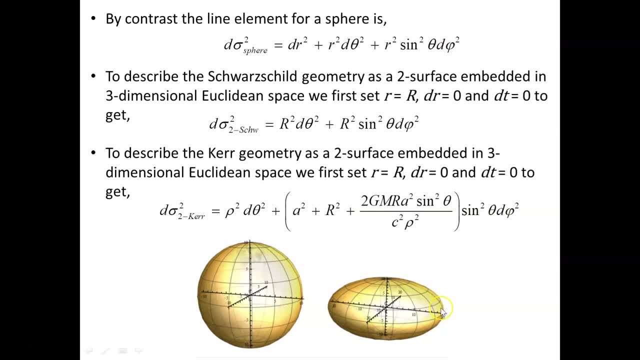 if you like. okay, and two very different shapes. so the sphere is described by this and the axisymmetric ellipsoid is described by this. and notice, we still keep that point right here and we keep that point right here as well. so we keep that point right here. we didn't put that point. 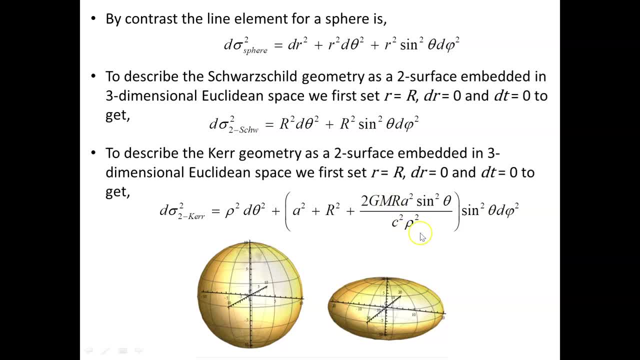 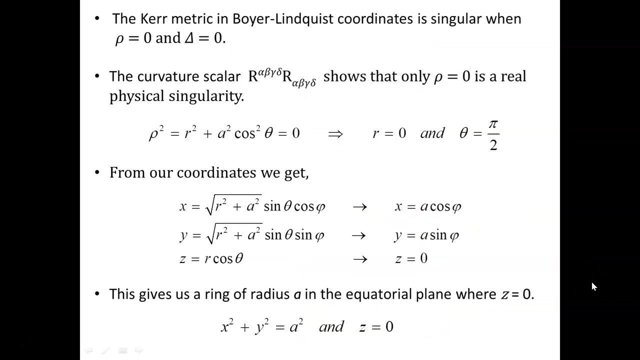 m term, the mass term, that plays a factor as well. okay, they're two very different highly symmetric sphere and the axisymmetric, which is symmetric around the axis for rotations, around the vertical axis here, but a very different shape to the sphere. that'll be important in the rest of the video. now, the Kerr metric and Boyer-Linquist coordinates is: 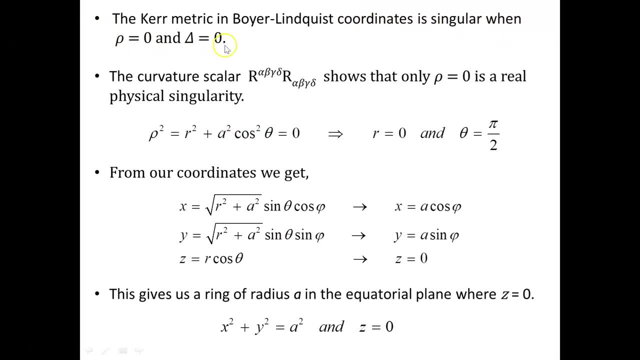 singular when rho equals zero and delta equals zero. um, i didn't put that in here now, just at: rho equals zero, the curvature scalar or the kretschmann invariant curvature scalar. kretschmann scalar or the invariant curvature scalar, this object here Riemann tensor with index. 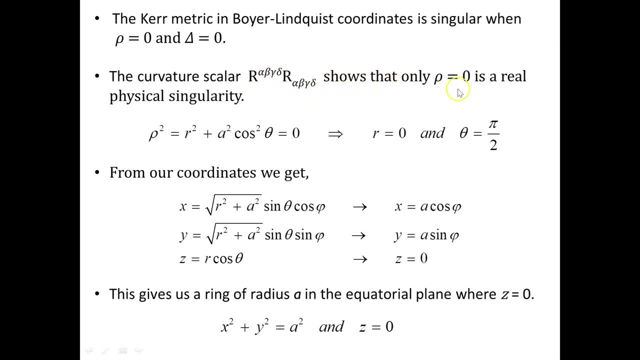 is up and all down. all applied together shows that only rho equals zero is a real physical singularity. now that'll be subject to the separate video. i don't need to go into that here. that is a separate video i'll go into, just as i did for the Schwarzstahl case. 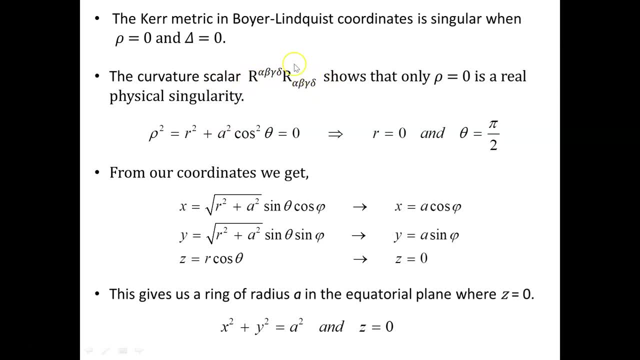 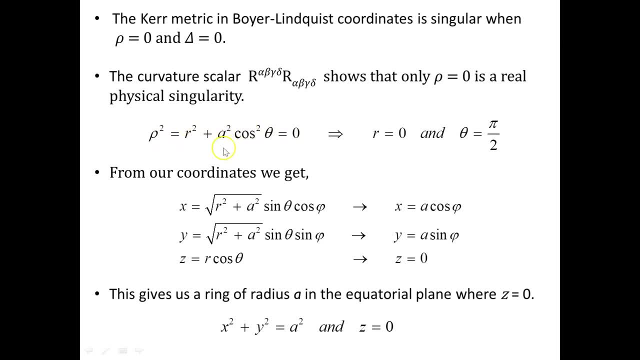 cos squared theta is zero. well, that employs uh implies to solve that we need r equals zero and theta it was pi on two. cos of uh. pi on two is zero and cos squared of zero is zero, and so this all goes to zero. for this condition now, from our coordinates we get. these are the coordinates: 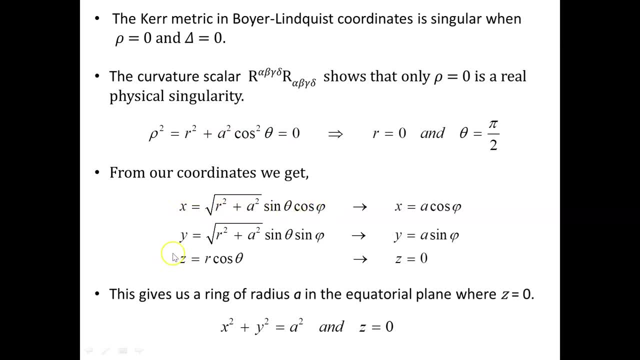 that specify the um axisymmetric oblate, ellipsoid. and if we set r to zero and we set theta to pi on two, um sine pi on two is one, sine pi on two is one, and what we get is r is zero. in here we get square root of a squared, which is a. so we get x is a cos phi. 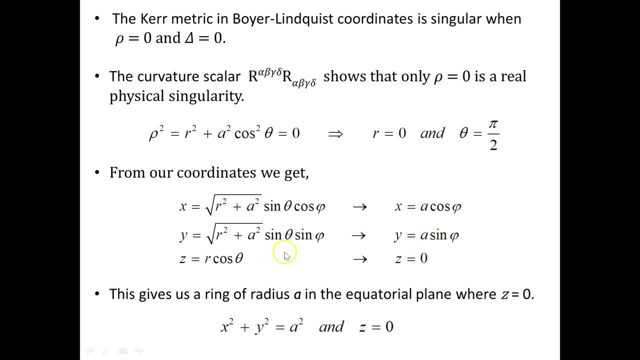 and here we get y equals a sine phi, because r is zero sine pi. on two is one, and so we get y equals a sine phi, and here r equals zero, so z equals zero. so what we've got? this gives us a ring of radius, a, um. these are polar coordinates in the equatorial. 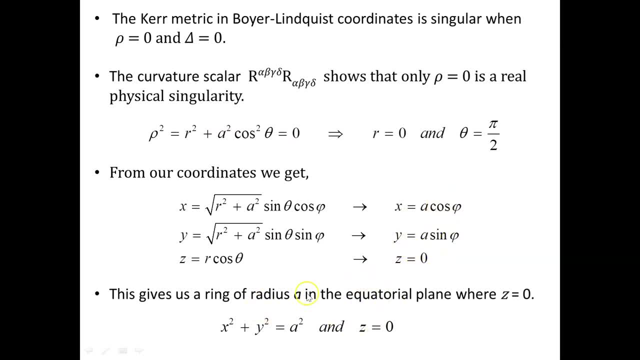 plane. in the xy plane it's a circle, um gives us a ring of radius a in the equatorial plane, where z equals zero, because that equals zero tells us we're in the equatorial plane, and so we have x squared plus y squared is a squared and z equals zero, and so that gives our first hint of what's. 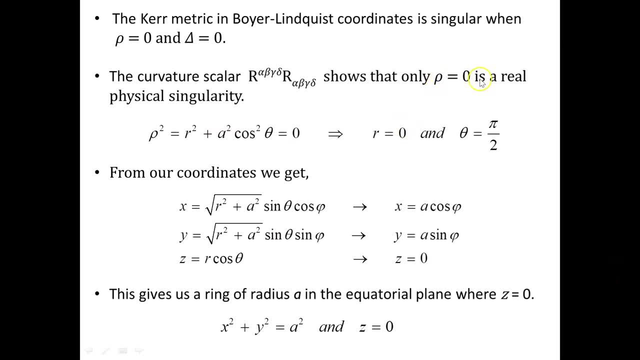 going on in the curve geometry, the phase of r is zero. and then for the curve geometry, we take the fact that rho equals zero is a singularity, and it's a real physical singularity, as the kretschmann scale will indicate. it blows up at that point. 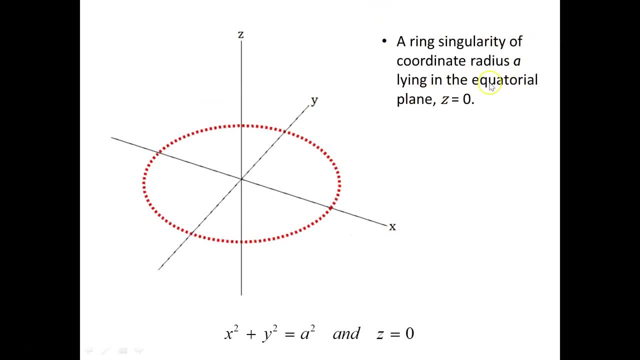 okay, so a ring singularity of coordinate radius, a lying in the equatorial plane: z equals zero. here it is okay. in the schwarzschild case our singularity was a point at r equals zero, which was here in our coordinate system. but in the kerr geometry our singularity is a ring. 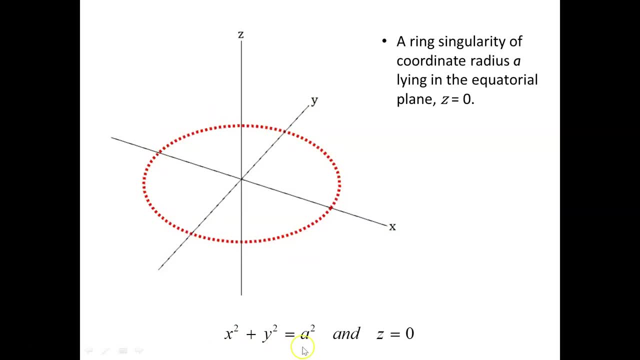 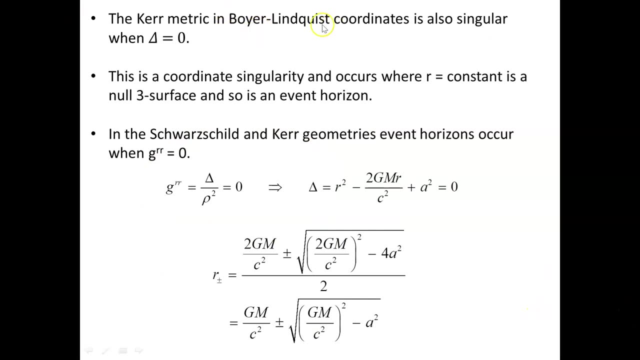 it's a ring of points of radius, a very different to the schwarzschild now the kerr metric and boya linquis coordinates is also singular when delta equals zero. this is a coordinate singularity that occurs where r equals constant, is a null three surface and so is an event horizon. 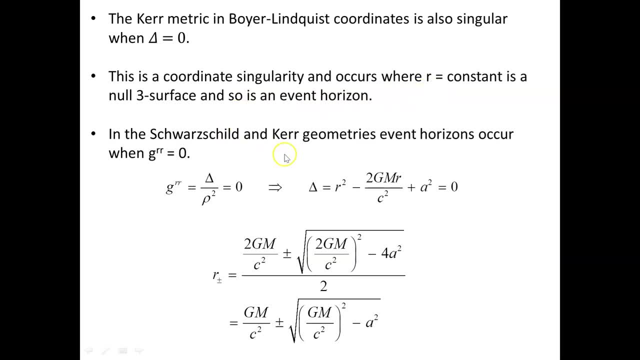 okay, so we set r equals constant. in the schwarzschild and kerr geometries, the event horizons occur when grr equals zero. if you have a look at the normal vector to the surface, there being a null surface, the null vector there helped us to locate that. and when we do that, 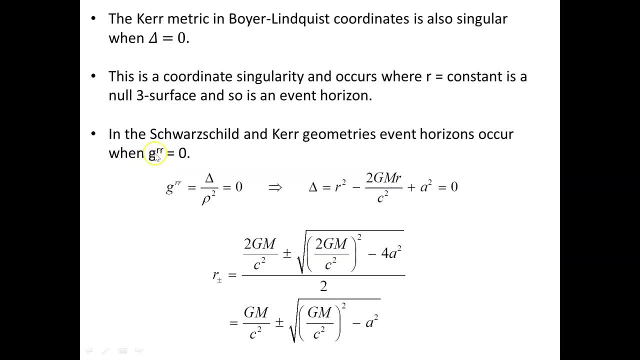 if you look at the previous video, number four in this series, you'll see that we require g contraverin rr from the inverse metric to be z zero For the Kerr metric. GRR is delta on rho squared equals zero. So multiplying through by rho squared implies that delta equals that object is equal to zero. 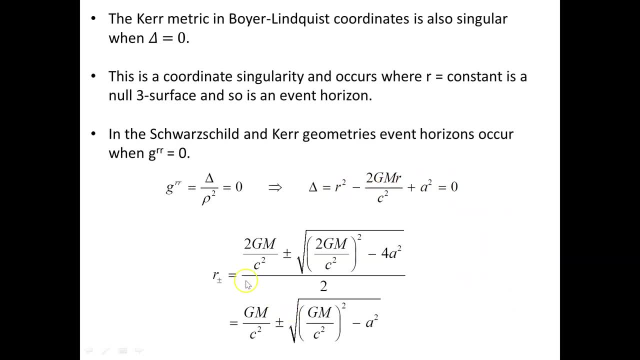 And when we solve that using the quadratic rule, we get two solutions here Plus minus this object in here. A little bit of algebra gives us this, So we've got two solutions. There are two event horizons, Not one as in the Schwarzschild. 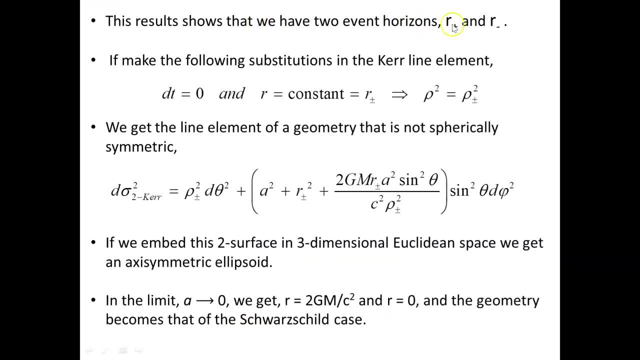 case but two. So we have two event horizons, one at R plus and one at R minus, And if we make the following substitutions in the Kerr line, element DT is zero, R equals a constant, which implies R equals R plus or minus, because 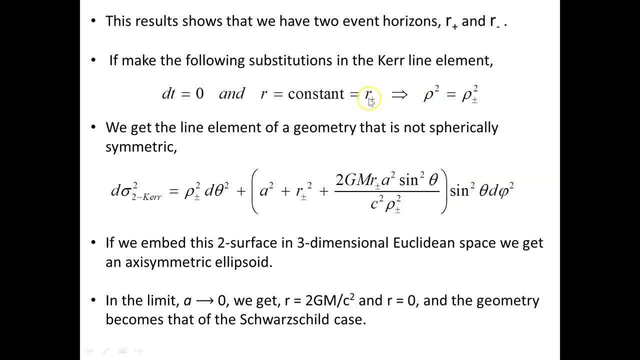 we're talking now about the event horizons. And what will the Kerr line element tell us Then, rho squared, is rho plus or minus? because, remember, rho squared had the R squared plus A squared constant. So R plus, R minus, hence the plus minus here. Now we get the line element of a. 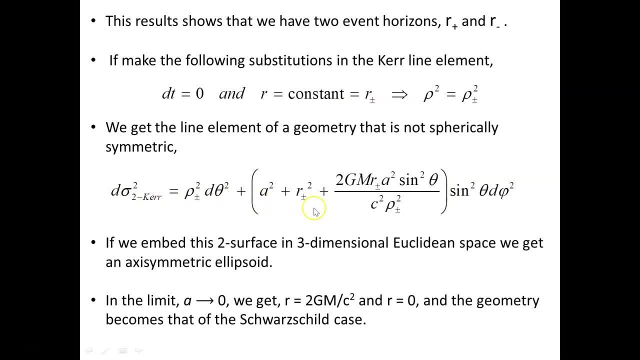 geometry that's not spherically symmetric. We've seen this right at the start of the video. This is not this two surface here described here. this two surface is not that of a sphere. If we embed this two surface in three. 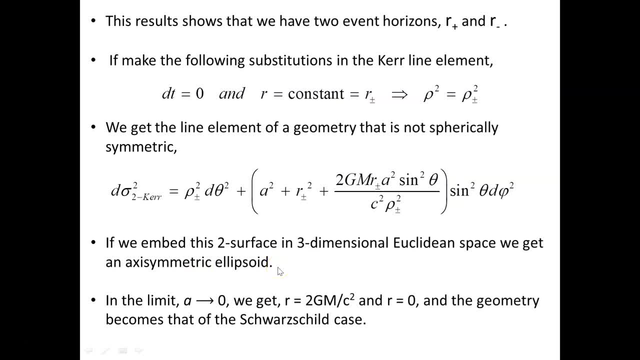 dimensional Euclidean space. we get an axisymmetric ellipsoid In the limit A approaches zero. Okay, We get R equals two GM on C squared and R equals zero And the geometry becomes that of the Schwarzschild case. So if A went to zero here, we would end. 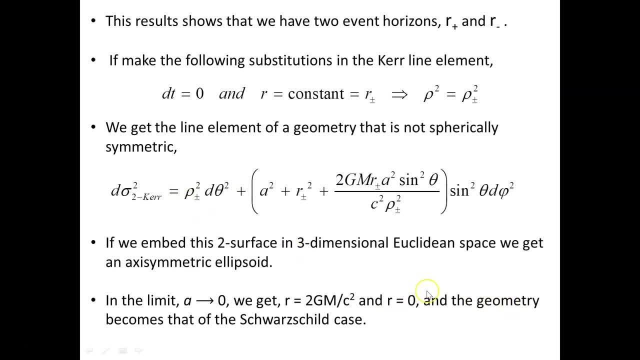 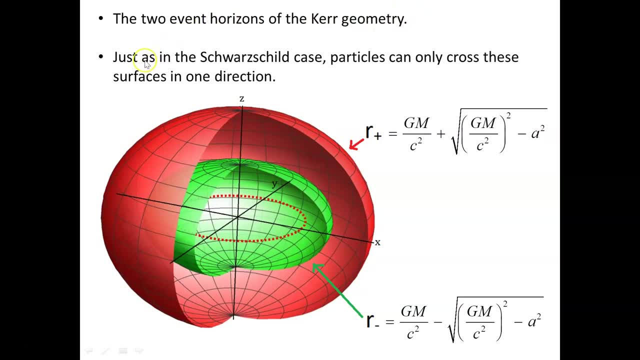 up with the case for the Schwarzschild spherical surface. All right, So the two event horizons of the Kerr geometry. just as in the Schwarzschild case, particles can only cross these surfaces in one direction. They are an event horizon. 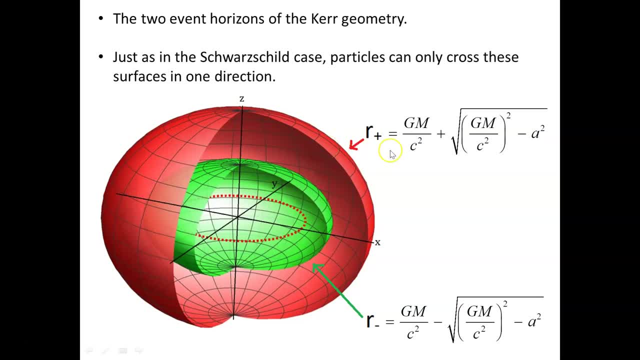 So in the last video they can only go in one direction and that's inwards. So R plus is the outer red surface here And R minus the outer event horizon, the inner event horizon. You can see here GM on C squared plus this object. 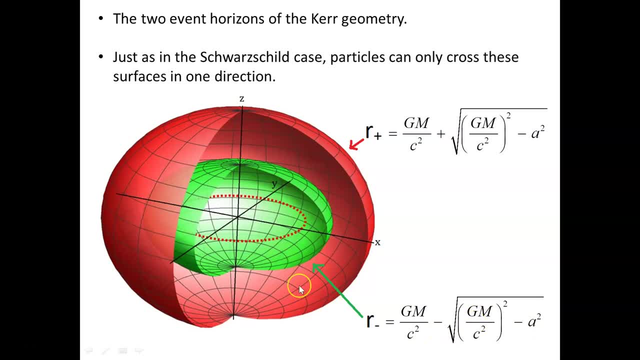 whereas GM on C squared minus this object here. And so here's our ring singularity in the middle. Here's our inner event horizon And here's our outer event horizon, The two event horizons Very different to the Schwarzschild case. 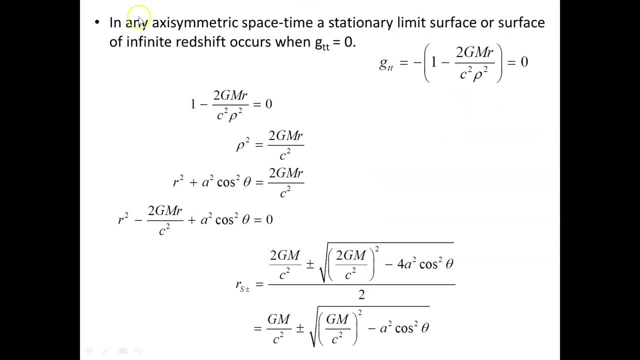 Okay. In an axisymmetric space-time, a stationary limit surface or surface of infinite redshift occurs when GTT equals zero. In the Schwarzschild case, this also gave us the event horizon. But in the Kerr case that does not. It gives us the 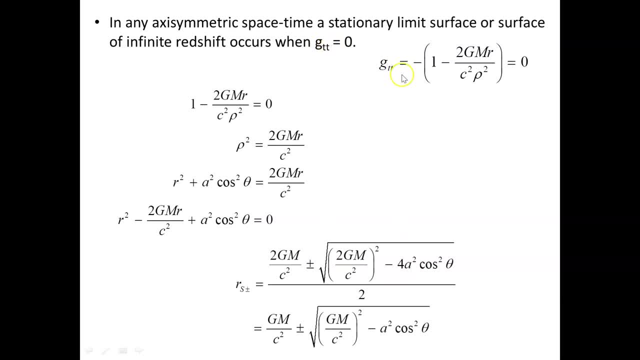 stationary limit surface or surface of infinite redshift. So GTT is this object here. We set it to zero, Solving it then. So multiply by minus one And then take the second term here on the right over on the left. sorry, second term on the left. 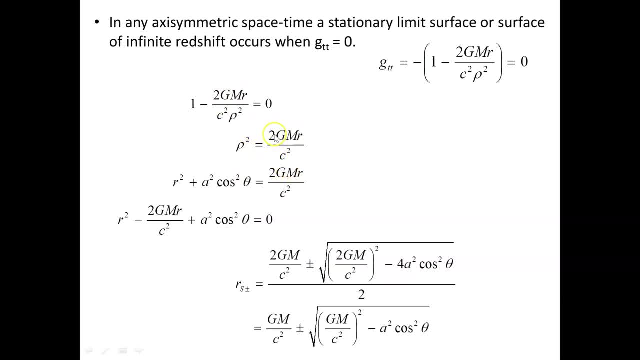 take it over to the right Multiply by rho squared. We've got this object here. Now rho squared is this: is that which is this business here? Okay, Now, this is the stationary limit surface, not the event horizon. Again, we apply the. 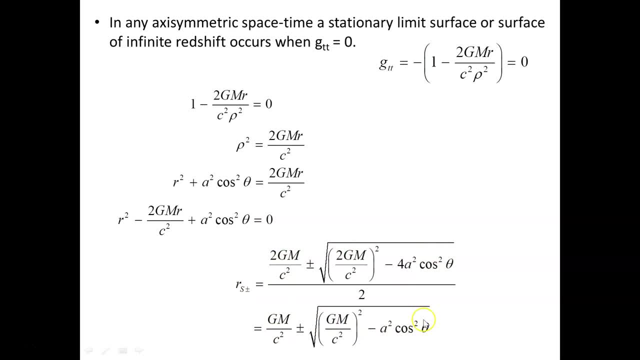 rule And there are two solutions here. A little bit of algebra tidies this up. Taking this under the radical becomes four, The two and the two cancel here. Taking it under the radical, two squared four cancels out. here Four cancels out. 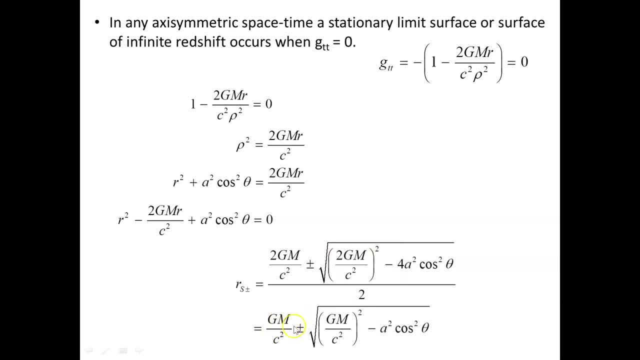 here And we're left with this object here. So there's two solutions. GM on C squared plus or minus the square root of everything under here. Okay, Now notice: in the event horizon there was no cos squared theta, Whereas in the, in the 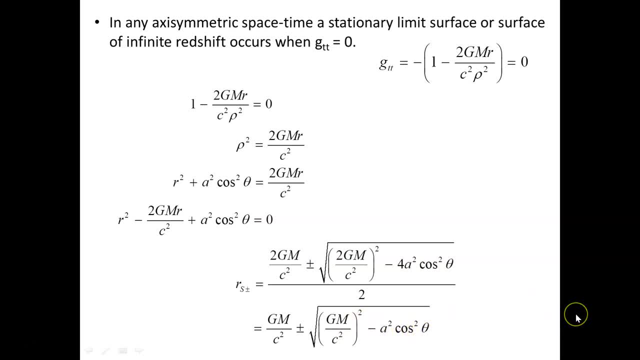 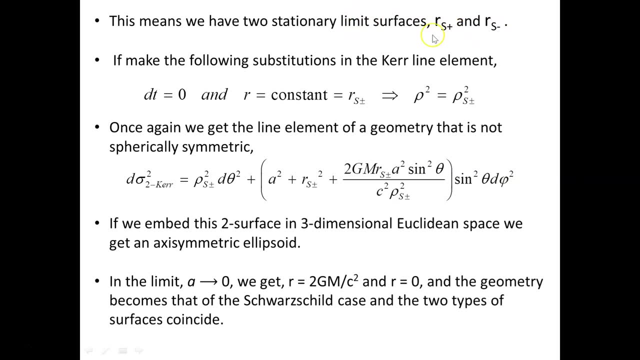 stationary limit surface. there is that cos squared theta factor. Okay, This means we have two stationary limit surfaces, R S plus and R S minus. Now if we make the following substitutions in the Kerr line element: DT equals zero, I equals constant, So we're producing a two surface And the 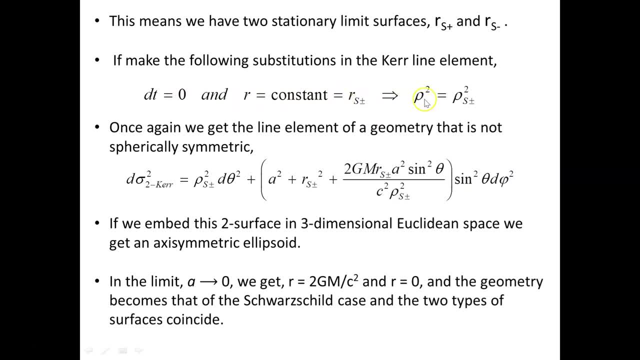 constant will be R S plus or minus either one of these surfaces. So rho square becomes rho squared, S plus or minus, given that rho contains an R square term and we're setting r to a constant. so once again, we let the line element of it. so once again, 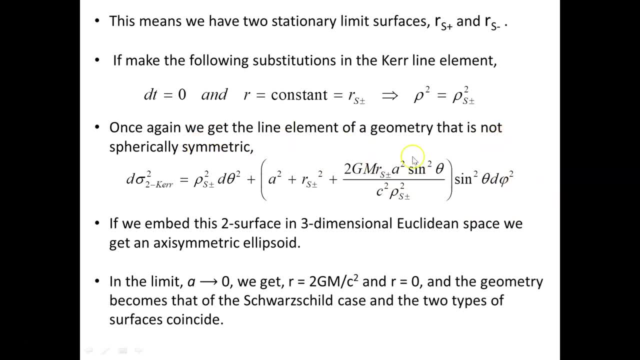 as we get the line on one of the geometry that is not spherically symmetric. this is not the geometry of a sphere. it's the geometry of an axisymmetric ellipsoid oblate, so dilated in the x and y directions and not in the z. if we embed this two surface in three-dimensional euclidean space, we 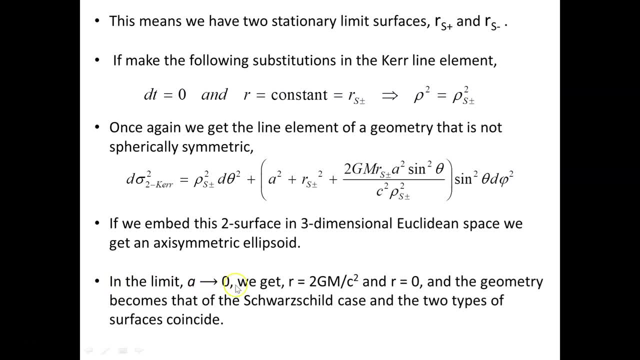 get an axisymmetric ellipsoid. again, in the limit a approaches zero, we get: r equals two gm, one c squared and r equals zero, and the geometry becomes that of schwarzschild case. so that rotation factor a, that rotation, that angular momentum per unit of mass times c is a very important factor because in 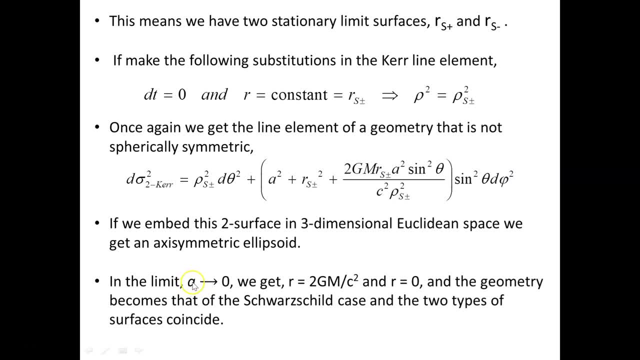 the schwarzschild case. obviously you don't have that, and so a equals zero takes us back to the schwarzschild case, and when that happens, these two types of surfaces coincide. once we take a to zero, the two surfaces, s plus, s minus, coincide, and they coincide with the event. 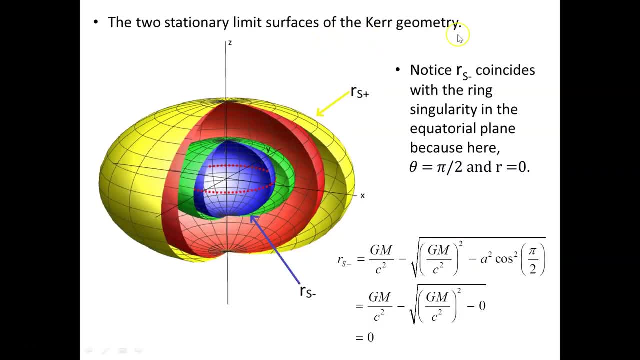 horizon. all right, so the two stationary limit surfaces of the kerr geometry, the yellow one here is the outer one and the blue one here is the inner one. and just notice a, the red one was the inner event horizon and the red one was the outer event horizon. 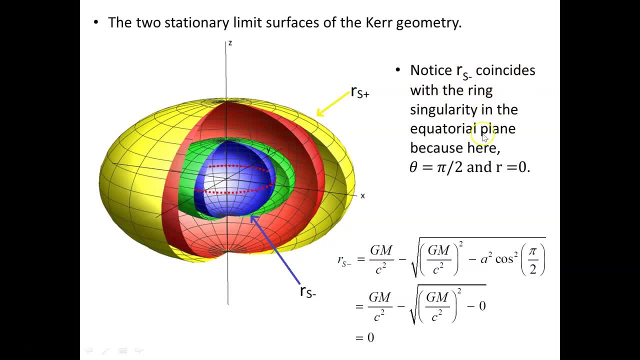 and notice: rs minus coincides with the ring singularity in the equatorial plane, because here theta equals pi on two, r equals zero. so rs minus is this object here. so in the equatorial plane theta is pi on two, cos of pi on two is zero. so cos squared of zero, zero. 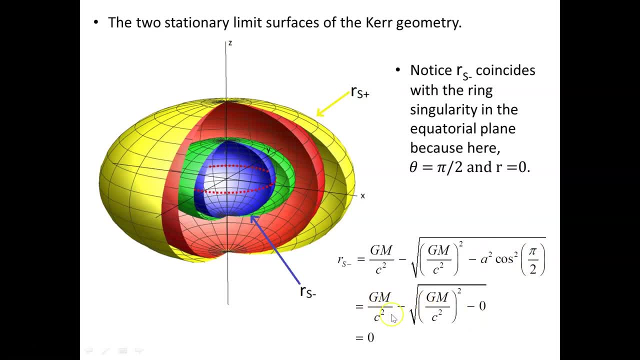 that drops off. we're left now with gm on c squared minus the square root of gm on c squared, all squared, which means they cancel out. we go: rs minus is zero, r equals zero and theta equals pi on. two was at the start of near the start of the video, was our solution and gave us the ring. 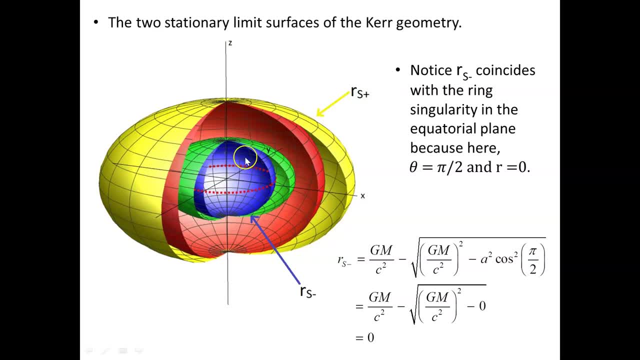 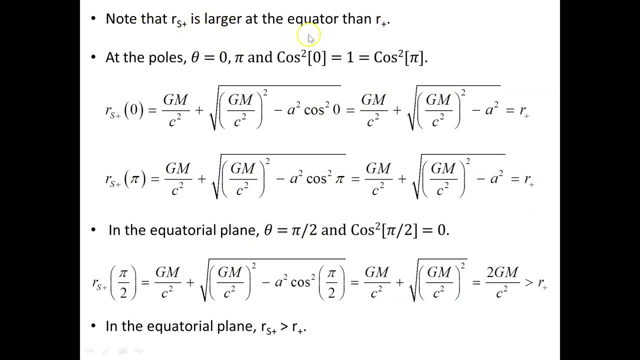 singularity in the red bit. so the inner stationary limit surface coincides with the ring singularity here. hence that's what's shown here. okay, now note that rs plus is larger at the equator than r plus. remember, this is the stationary limit surface, the outer stationary limit surface. 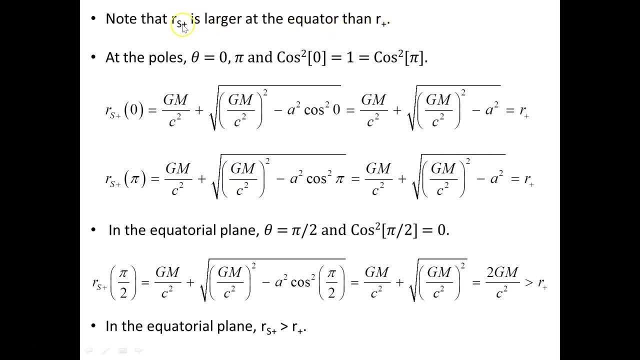 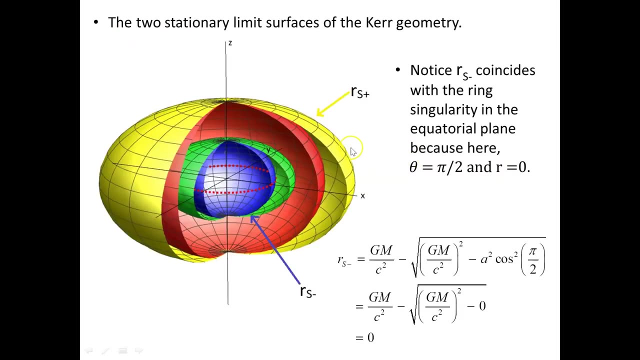 and this is the outer event horizon and that is the outer stationary limit surface encompassed within it, the event horizon r plus. so can we check that that's actually the case now at the poles? if i go back a bit at the poles, we're saying these two are the same. 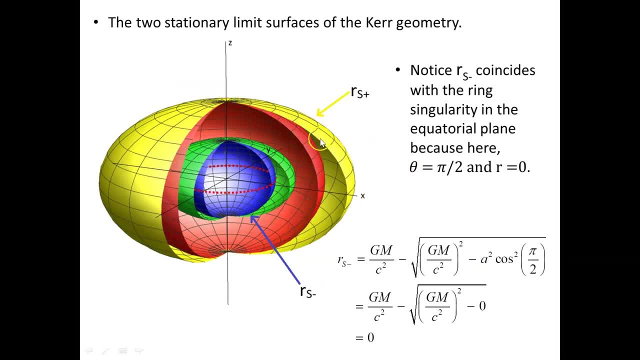 okay, here's the outer event horizon, here's the outer stationary limit surface. we're saying they're the same at the pole, so we'll check that in a minute. and then we're saying that the stationary limit surface extends past the event horizon at the equator. so we're going to. 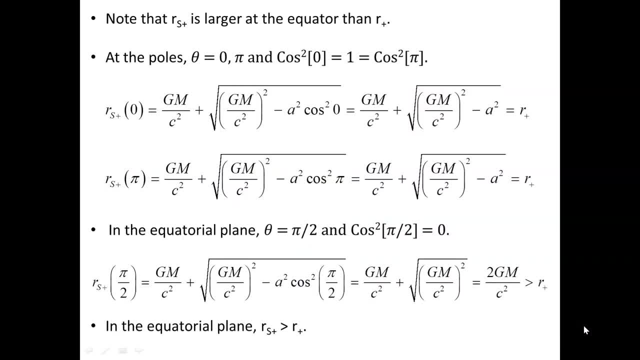 check that. that's at pi on two. all right, so at the poles, theta equals zero, l pi pole is zero, southern pole is pi, and cos squared of zero is one and cos squared of pi. cos of pi is negative one, but squared is plus one, so both of these are equal to each other. to the 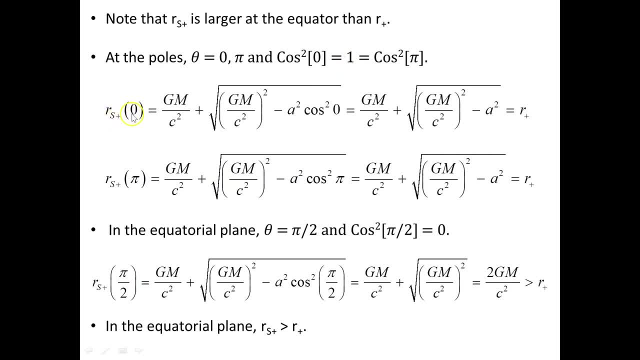 value of plus one. now, the stationary limit surface at theta equals zero, gives us this object here, which is this, and that is just the event horizon at theta equals zero. at pi, the southern pole, again the same thing. okay, this will come to one, and so we get this object here. okay, again, which is r plus. 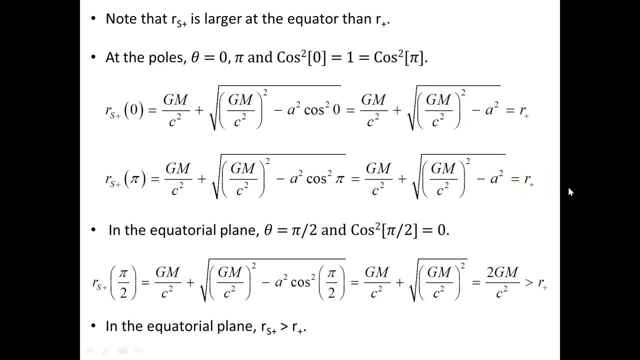 so at the poles the stationary limit, surface and the event horizon coincide. they share the coincidence at the same point. let's have a look in the equatorial plane now. theta equals pi on two, and here, cos squared pi on two is zero. cos of pi on two is zero, square is still zero. 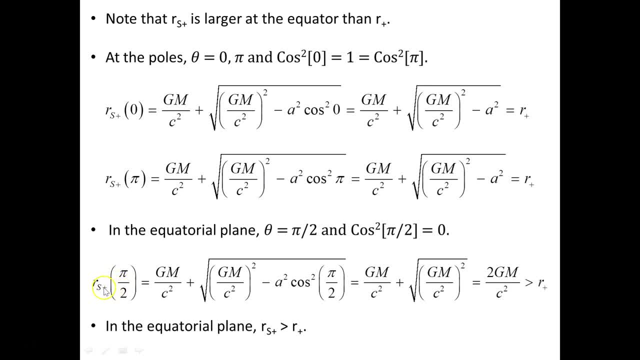 so rs plus the outer event, the outer stationary limit surface. sorry at pi on. two, is this object here? we've seen that this here is zero, so that drops out, and what we're left with is gm on c squared plus the square root of gm all over c squared, all squared, and so we end up with two of these. 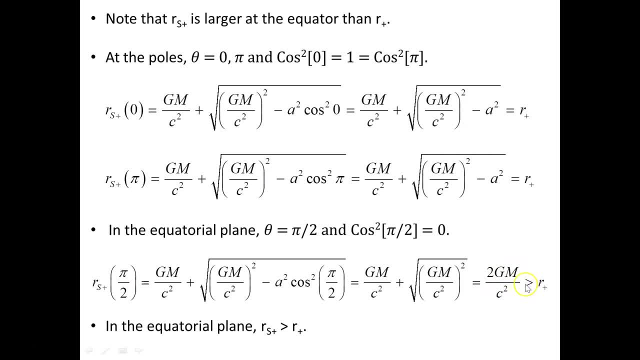 two gm on c squared and that is greater. 2gm on c squared is greater than the outer event horizon. and where the outer event horizon is this object, here gm on c squared, one of them, not two of them, plus the square root of this object here. 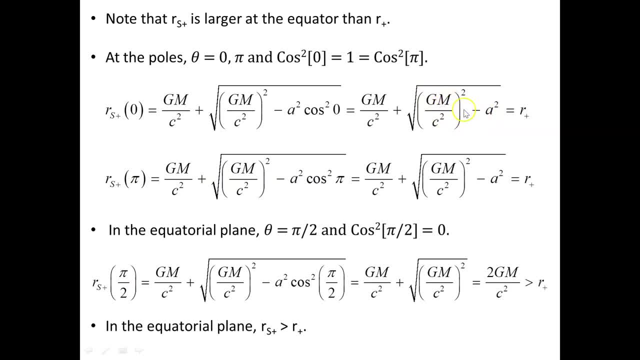 minus this bit. so if we take this away and take the square root of it, it's going to be smaller than just gm on c squared and so, and so what happens is that this works out to be less than this. so in the equatorial plane, the stationary limit surface. 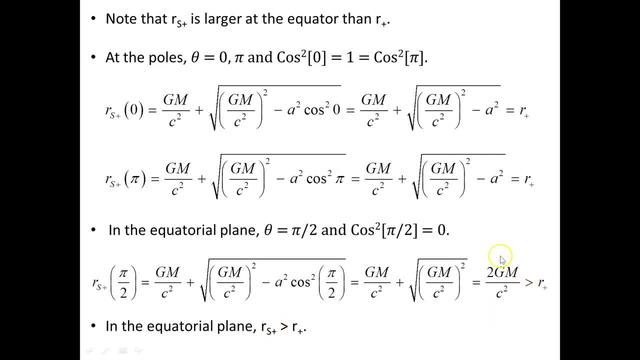 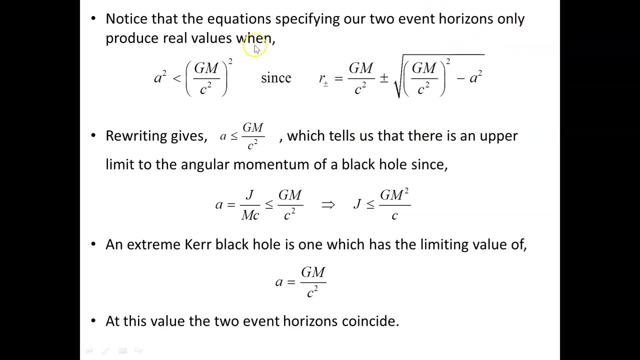 passes outside, beyond the event horizon, and we can see that clearly. this is greater than all of this. all right, notice that the equations specifying our two event horizons only produce real values when a squared is less than gm on c squared. so here, when a squared here is less than this, we're taking the square root of a positive quantity or zero. 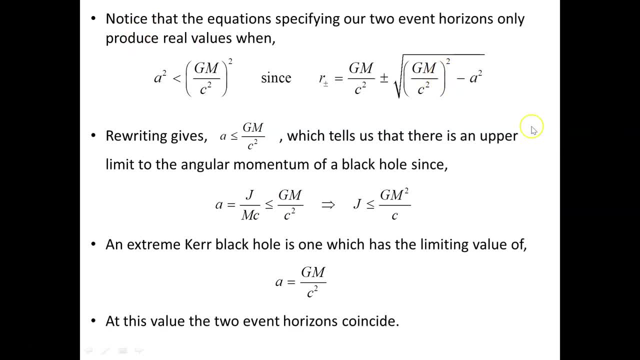 and so what happens? what happens here is that this is produces real values. if this were equal to- and i thought i'd change that- so if a squared is equal to or less than when these two are equal, this is zero. we still produce a real value. um, now rewriting gives a is equal to less than gm on c squared. 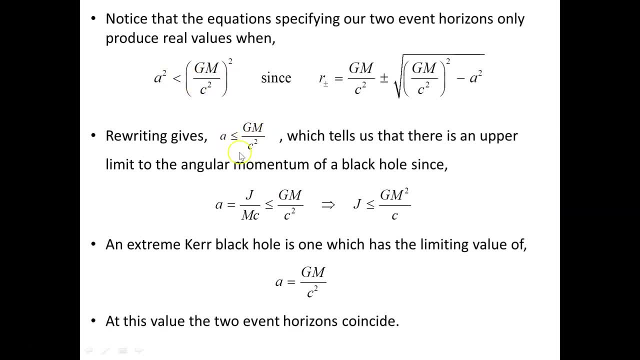 um we can take the square root of both sides there gives us this: we don't change the direction of the inequality here. and that tells us that there is an upper limit to the angular momentum of a black hole, rotating black hole. since um a is g on mc, okay is equal. 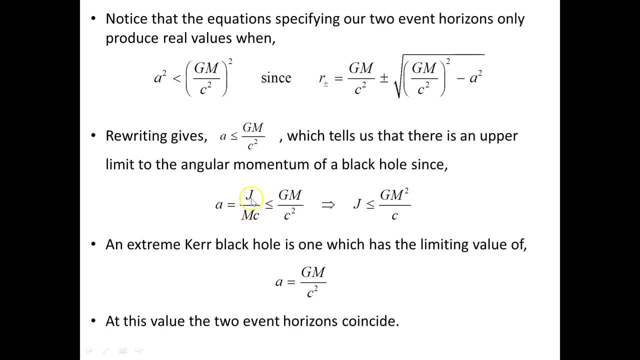 to less than gm on c squared, as we've seen now here. let's just multiply through by m. okay, we get gm squared over all right now. these are positive quantities, so we can multiply through and it doesn't reverse the direction of the inequality. and so the angular. 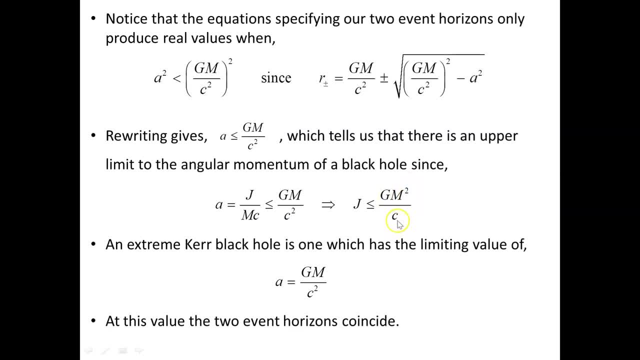 momentum is equal to less than gm squared on c, so there's a limiting value for rotating black holes of the angular momentum. okay, so there's a limit. an extreme curve black hole is one which has a limiting value of a equals gm on c squared. when we actually get a equal to this, that is a limiting. 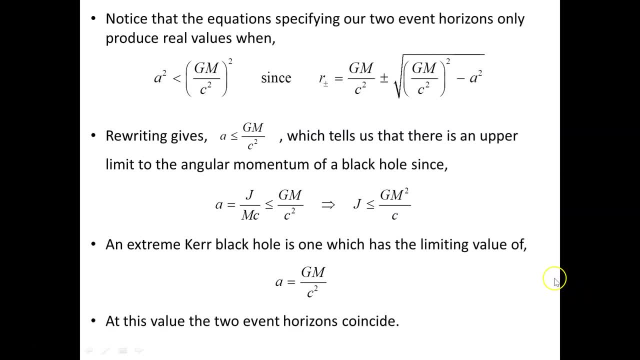 value. at this value, the two event horizons actually coincide, because if that squared is equal to that squared, they cancel out and we're just left with this value here, and which means that we get r plus and minus is just this value here. okay, so the two event. 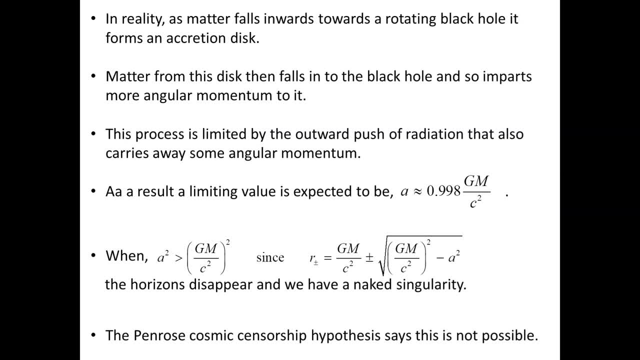 horizons coincide. in reality, as matter falls in towards a rotating black hole, it forms an accretion distance of gm squared on c squared, which is equal to less than gm squared on c squared. matter from this disc then falls into the black hole and so imparts more angular momentum to it. so 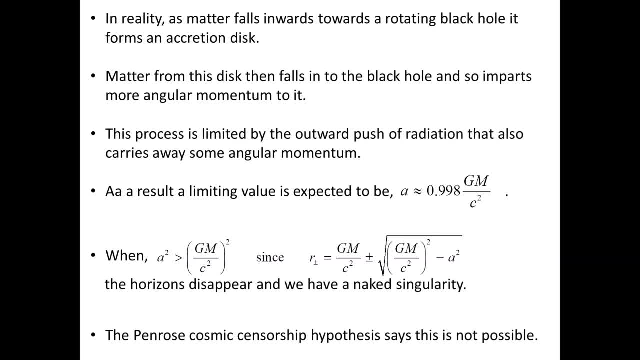 it can spin it up, increase its angular momentum, but this process is, uh, increasing its angular momentum- is limited by the outward push of radiation that also carries away some angular momentum. so there is a limiting value and it's, it's the combination of these two processes. the 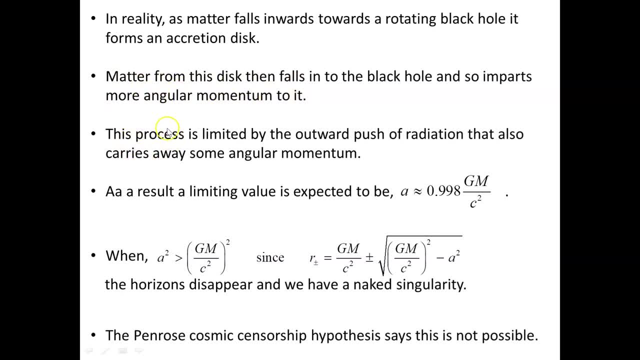 infalling matter, giving it angular momentum, and the radiation carrying away angular momentum um energy, and it carries away energy and angular momentum and so it acts to moderate the this process here. so you can't spin up a black hole to any value of angular momentum. there are limiting processes involved. 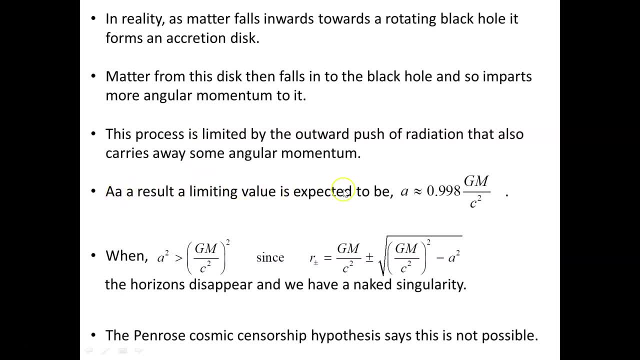 now, as a result, not aa, sorry. as a result, a limiting value is expected to be- and there are some calculations for this, but i'm not getting into that here for this video- but the limiting value is about 0.998 gm on c squared. uh, there are some examples of 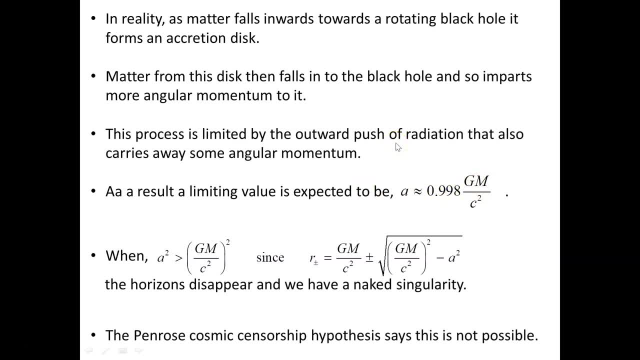 measurements performed that find this to be, uh, the angular mentor to be, i think, the highest. about one case i think it was about 74 percent of the maximum extreme value. so, uh, there are some quite uh uh black holes out, rotating black holes out. there was ex quite extremely high, uh, angular and 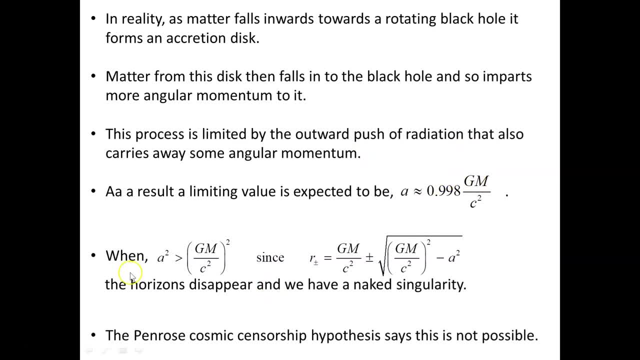 and i think that's the main reason why this is so important- but less than the maximum value. okay, now when a squared is greater, now watch out, when a squared is greater, so this bit here is greater than that, the horizons disappear and we have a naked singularity, because here we start. 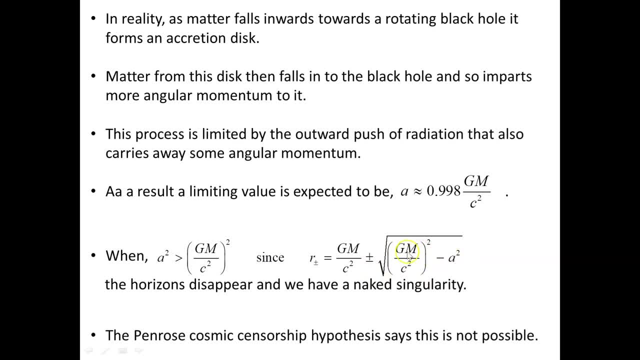 producing complex values. so minus a squared. if a squared is greater than this, you've got a square of a negative number here. now you start producing complex values, the horizons disappear and we have Now the Penrose Cosmic Censorship Hypothesis says this is not possible. 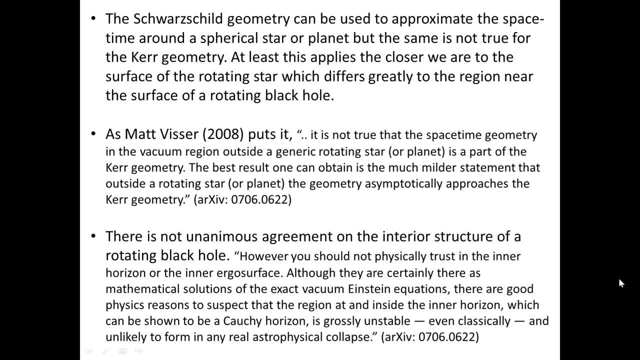 You won't have naked singularities. Okay, now, the Schwarzschild geometry can be used to approximate the space-time around a spherical star or planet, but the same is not true for the Kerr geometry. At least, this applies the closer we are to the surface of the rotating star. 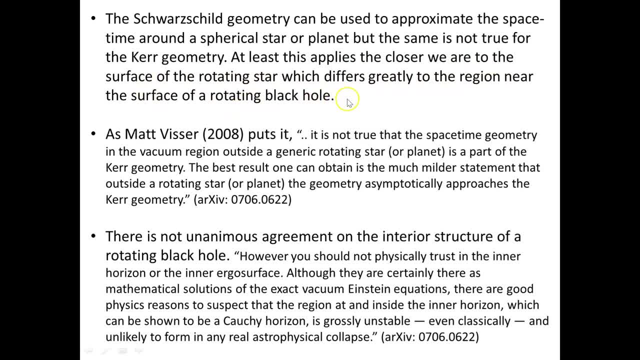 which differs greatly to the region near the surface of the rotating black hole. So although the Schwarzschild geometry with all its high degree of symmetry can be used to approximate a star or a planet, you can't do that when it comes to rotating. 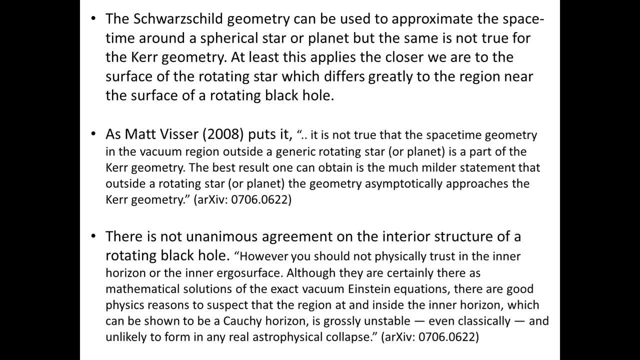 because, as we've seen in this video, the rotating black hole has a number of surfaces, a number of stationary limit surfaces, two stationary limit surfaces and two event horizons, and they don't approximate- Okay, They don't approximate- the surface of a star or planet. 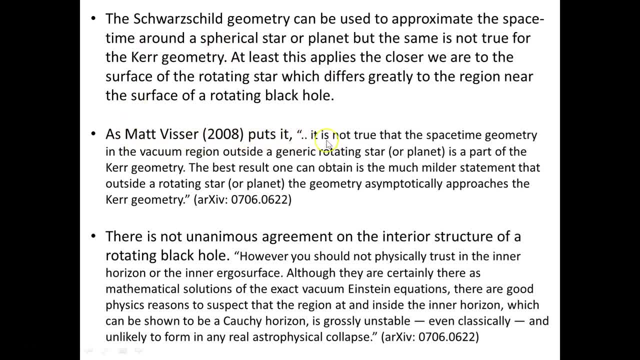 Now as Matt Visser 2008, puts it now. having said all that, it's not clear that all the content of this video is agreed on by everyone. There do seem to be arguments for some of the inner structure. 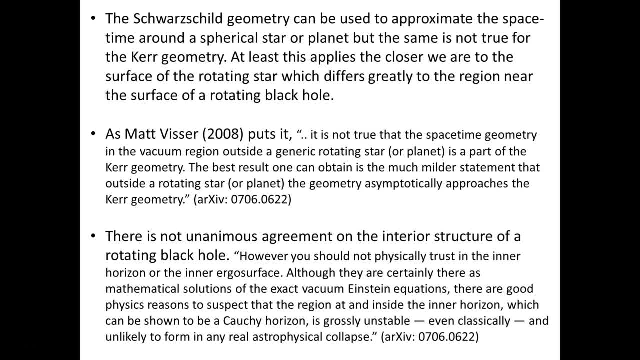 the inner event horizon and the inner stationary limit surface perhaps don't form, They're not stable enough in a rotating, rotating black hole, because, remember, in a rotating black hole the angular momentum adds to the energy, which in turn creates its own gravitational field. 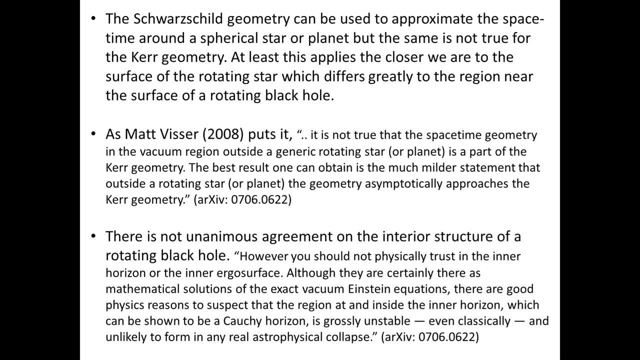 Unlike in the Newtonian case where it doesn't, anything that generates energy and so on has its own: the energy itself that generated then has its own gravitational field and it feeds into it. So whether or not a structure like shown in the video would form or not is not entirely clear. 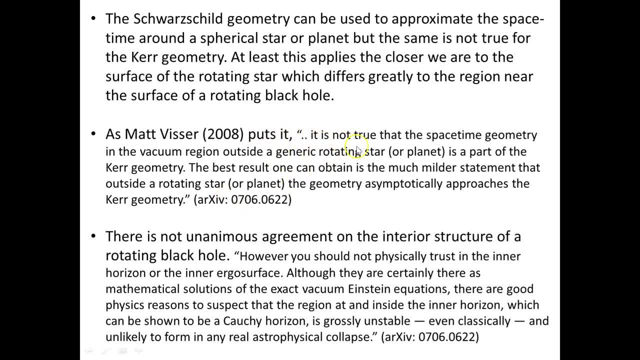 Not everyone agrees. So, as he puts it in his paper here, it is not true that the space-time geometry in the vacuum region outside a generic rotating star or planet is a part of the Kerr geometry. The best result one can obtain is the much wildest. 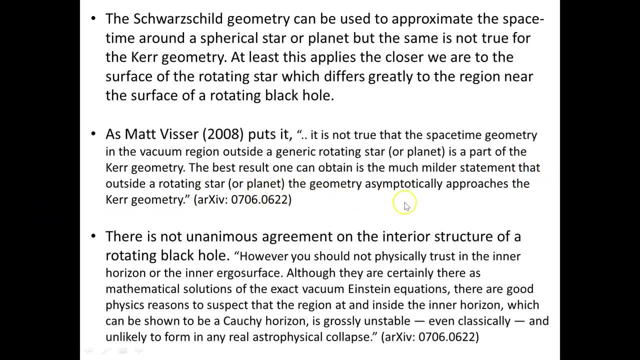 milder statement that outside a rotating star or planet the geometry asymptotically approaches the Kerr geometry. So at best you can't really use. you can't really use the Kerr geometry to approximate a rotating star or a planet, except perhaps in the asymptotic limit as you move further and further away. 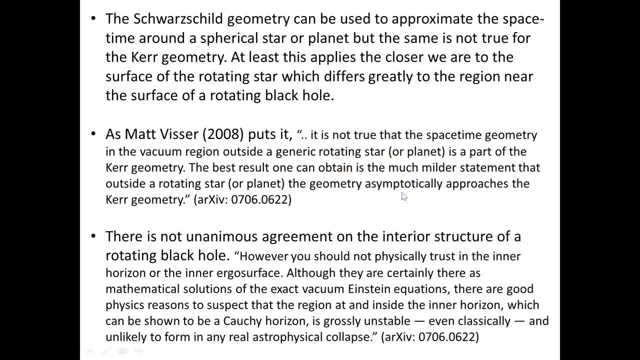 I mean with a rotating star or planet, you're still going to have frame dragging. It would be extremely mild- The gravity B probe was trying to look at that, but very mild Anyway. his paper I'll include in the description below the video. 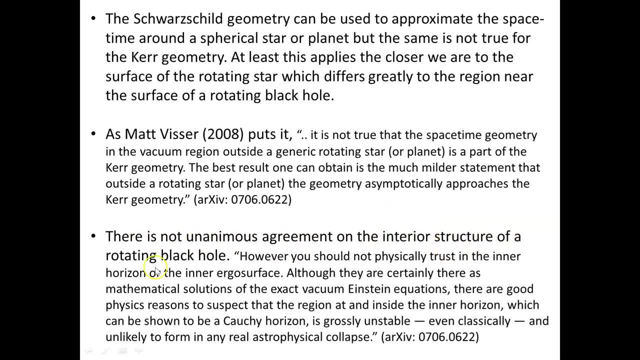 Now there is not unanimous agreement on the interior structure of a rotating black hole. Again from Matt Visser. However, you should not physically trust in the inner horizon or the inner ergo surface, meaning the stationary limit surface, although they are certainly there as mathematical solutions of the exact vacuum. Einstein equations: 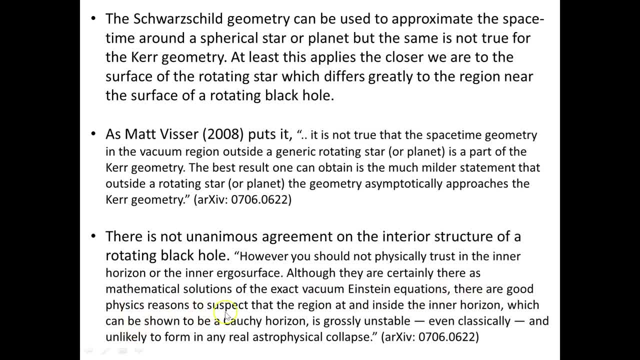 There are good physics reasons to suspect that the region at and inside the inner horizon which can be shown to be a Cauchy horizon stationary limit surface is grossly unstable, even classically, and unlikely to form in any real astrophysics collapse. 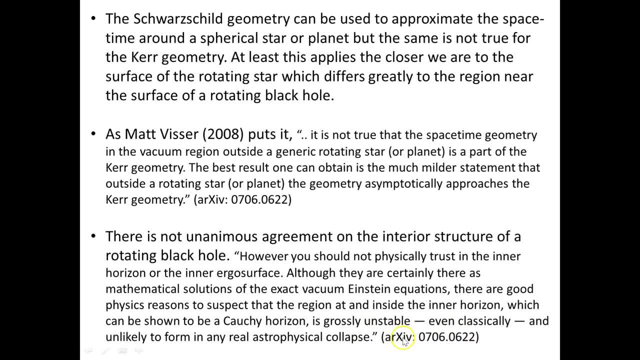 So again, this comes from the same paper there. So there's not unanimous agreement that these structures form something that I do mathematically, but whether or not in a real physical situation I would. perhaps it's too unstable. The angular momentum and other factors feed back into the, you know. 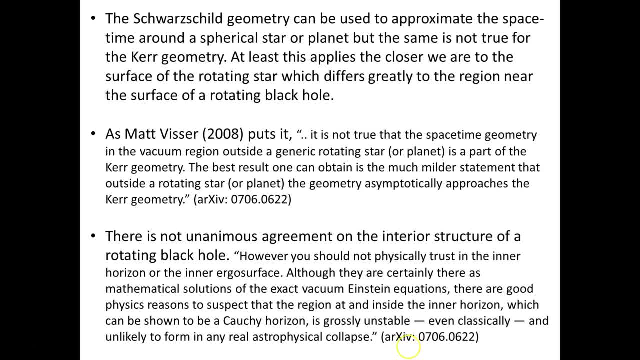 the field, equations, feedback into the field. whether or not, it's not entirely clear, even though mathematically it appears to be clear. So this paper I'm going to include in the video description below. One more thing now, just the structure of the Kerr black hole. 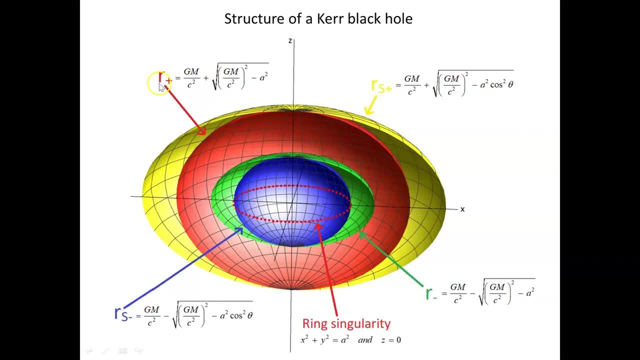 So what we found in this video here is that the outer event horizon, the red one, here, the outer stationary limit, or infinite redshift surface in yellow here and then in here we have the inner event horizon, the green, the ring, singularity of red and the inner stationary.